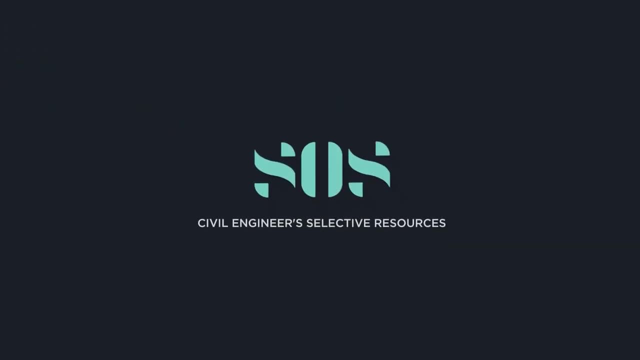 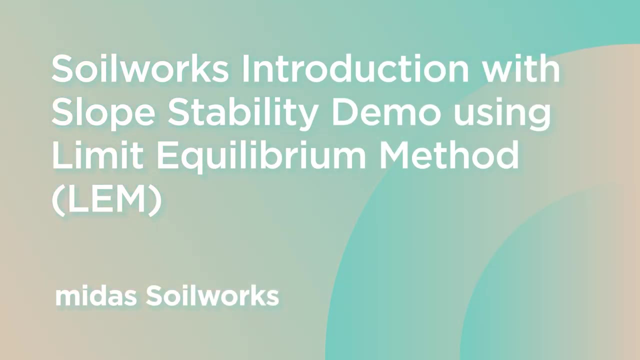 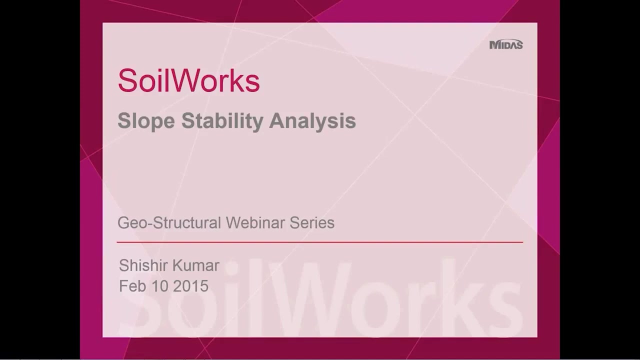 Hello everyone, welcome to this session on Slope Stability Analysis using Miner Soilwork. In the last session we discussed about the usage of Midas Civil for box culvert and RC slab bridges and understood that checking the stability of slopes near the structure is as important as designing the structure itself. 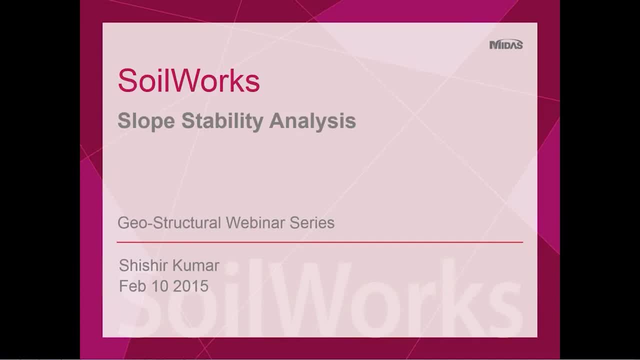 To deal with any sort of slope stability problems. Midas provides GTS-NX and Soilworks. GTS-NX is a 2D and 3D FEA software, whereas Soilworks is 2D only with analytical methods supported, along with finite element analysis methods. 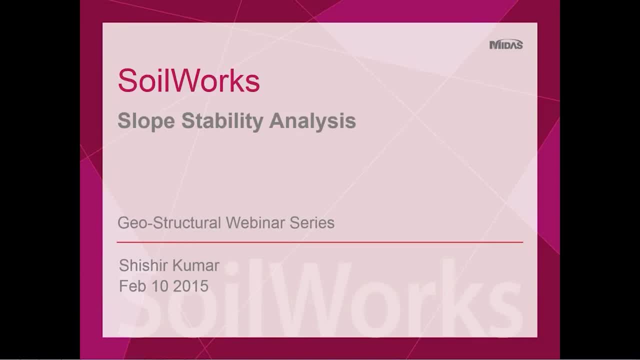 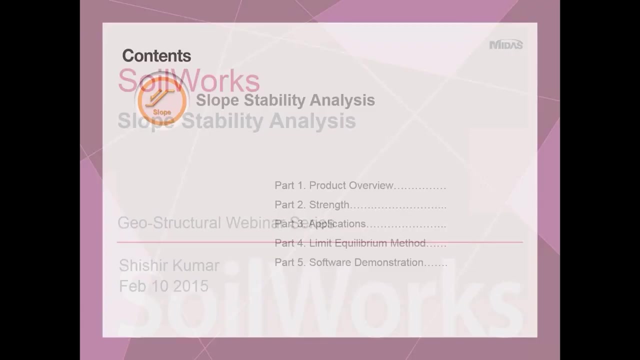 One such analytical method most commonly used for slope stability analysis is Limit Equilibrium method, which is the topic of our today's discussion. This is how I am going to proceed. Firstly, I will give a product overview. Then I will discuss the strengths of Midas Soilworks. 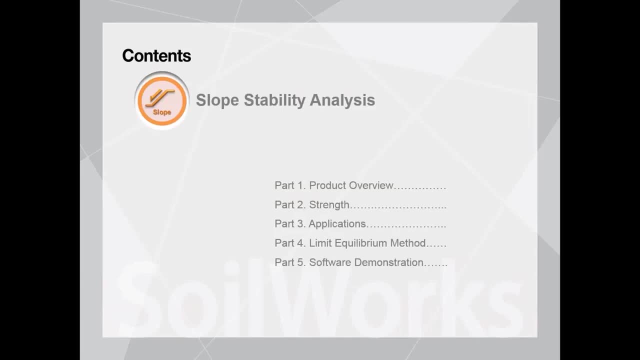 Then applications of Midas Soilworks will be discussed. Next Limit Equilibrium method, its theoretical background and applications of Midas Soilworks. Next Limit Equilibrium method: its theoretical background and applications of Midas Soilworks. Next Limit Equilibrium method: its theoretical background and applications of Midas Soilworks. 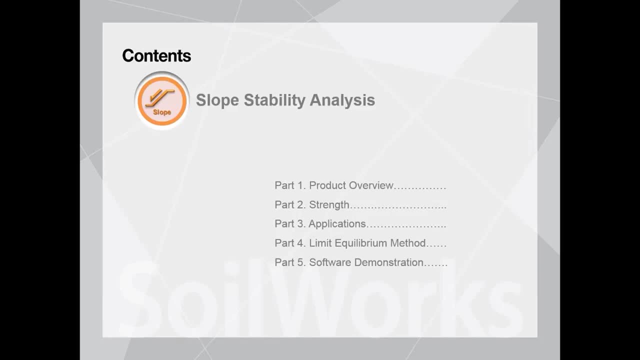 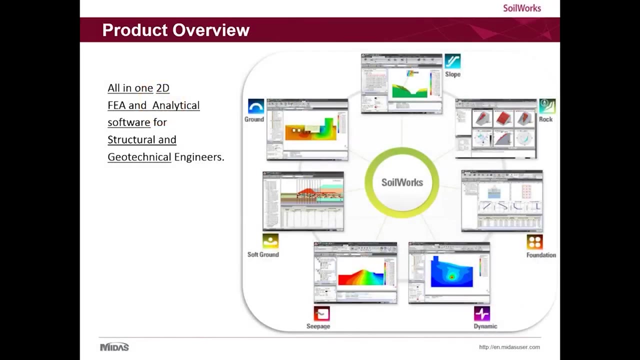 The software demonstration on Limit Equilibrium method for slope stability analysis will be followed. Let me give you a product overview. Midas Soilworks is all-in-one 2D FEA and analytical software. Midas Soilworks is all-in-one 2D, FEA and analytical software. 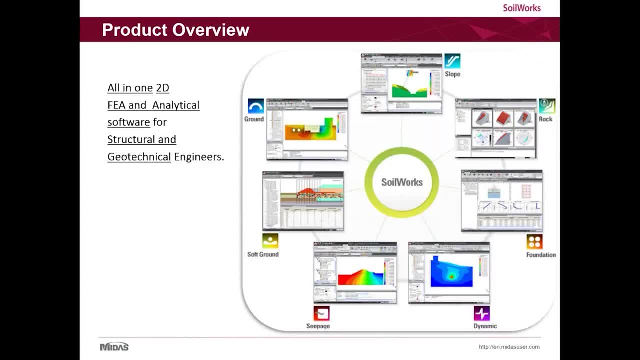 Midas Soilworks is all-in-one 2D FEA and analytical software and geotechnical engineers. it has seven modules. first is slope module for slope stability analysis using strength reduction method, stress analysis method or limited equilibrium method. other is rock module, which is a module for 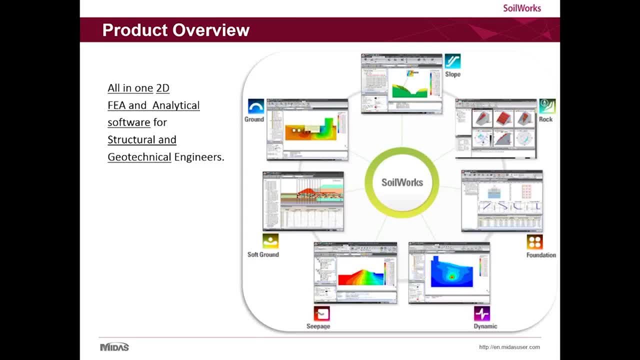 failure modes, slope stability and various other analysis on rocks. third is foundation module for py analysis for various configurations of files. fourth is dynamic module, which is for seismic analysis with a huge database for time history records of major earthquakes. fifth is seepage module, which is to 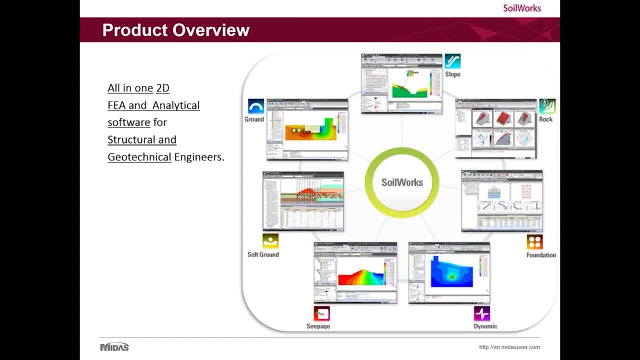 analyze the effects of seepage. it's mainly for dams and levees but can be used in other cases also for to determine the pore water pressure soil works. sixth module is soft ground module, which is for immediate settlements in sandy soils or consolidation settlement in clay soils over long pj. last is ground module, which 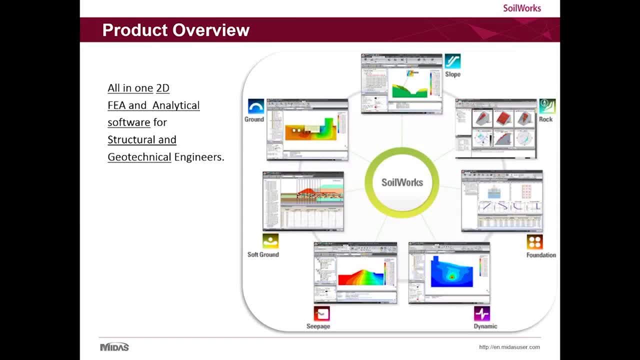 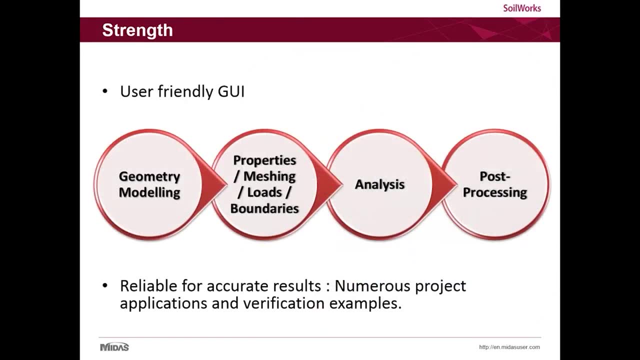 is mainly for tunnel analysis, but can be used for analyzing the effects of cutting and filling. if you see the workflow of any finite element analysis software, it would be as shown on your screen. first is we have to model the geometry. next we have to define the properties, mesh the structure, define the. 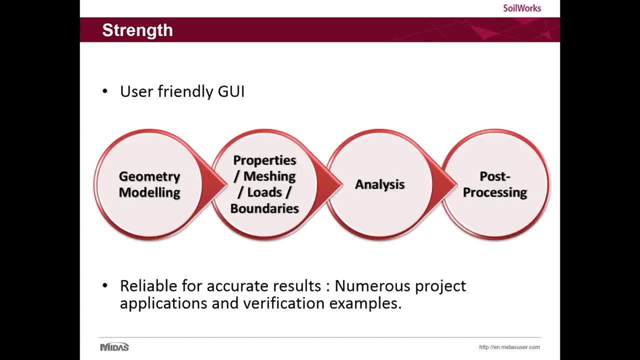 loads, define the boundary conditions, then run the analysis and then check the post-processing results. GUI of minor soil works is so user-friendly that to follow this workflow you just have to move from left to right for modeling of the soil work process. G-U-I of minor soil works is so user-friendly that to follow this workflow you just have to move from left to right for modeling the soil work process. 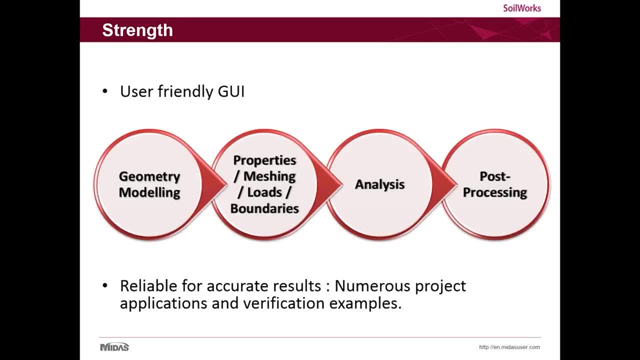 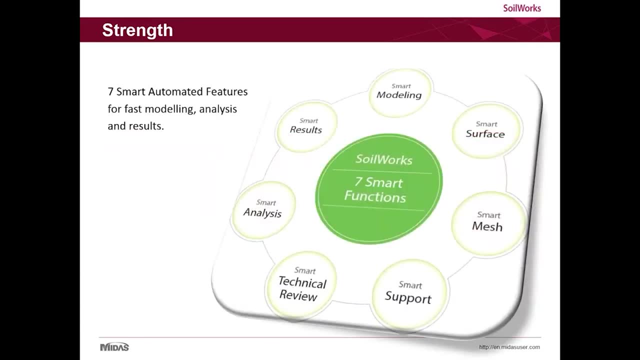 in obtaining the results, So the entire operation becomes very intuitive. Soilworks is reliable for accurate results and we can say this because of our numerous project applications and verification examples. Soilworks has 7 smart features and I will discuss these in detail in the next slide. 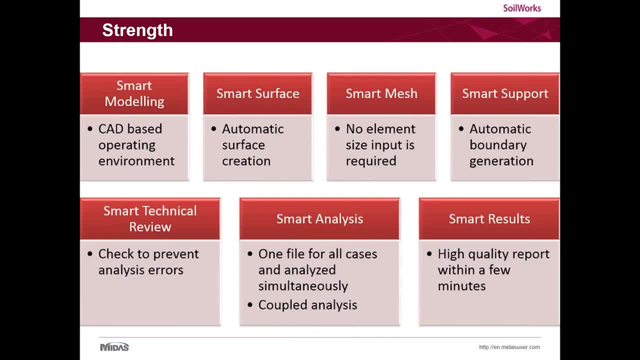 First is Smart Modeling, which is CAD based operating environment. In Midas Soilworks, we can import any CAD geometry and perform the modeling on it, or it has CAD based options using which we can edit the model. Next smart feature is Smart Surface, which creates a 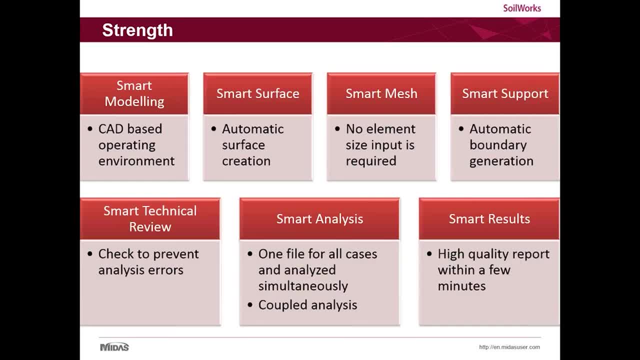 surface quite quickly, within few seconds. Third is Smart Mesh, for which no element size input is required, So anyone without in-depth finite element modeling knowledge can also use Soilworks, and the software defines the mesh best suited to get accurate results. Midas Soilworks provides smart support using which we can generate boundary conditions. 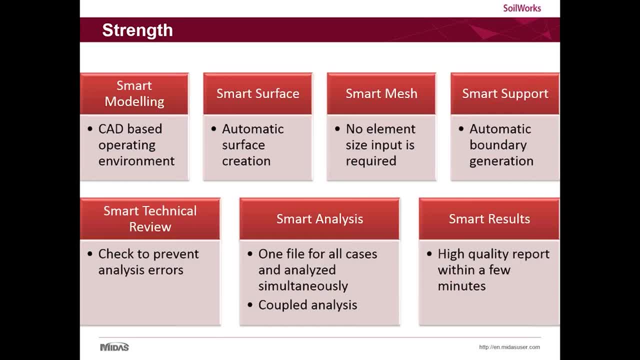 automatically. We will see all these smart features in the next slide. Soilworks is reliable for accurate results and we can say this because of our numerous projects applications. and we can say this because of our numerous projects applications And then see the results of our various projects projects. 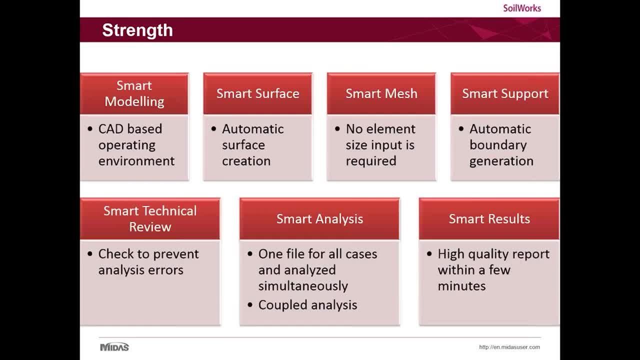 Next is Technical Review And using which we can check the definitions and janitority and prevent analysis errors. Next slide, and which we need just one file. we can analyze all of our analysis cases simultaneously. Soilworks also provides Coupled analysis, coupled analysis and Photoshop sense. 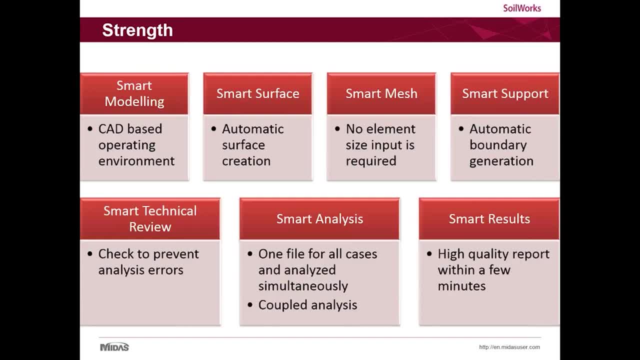 Coupled analysis is the case, like we can perform seepage analysis and get the results of pore water pressure and use it as a pressure inside the soil for slope stability analysis. So this kind of coupling is provided in with several modules of soil works. 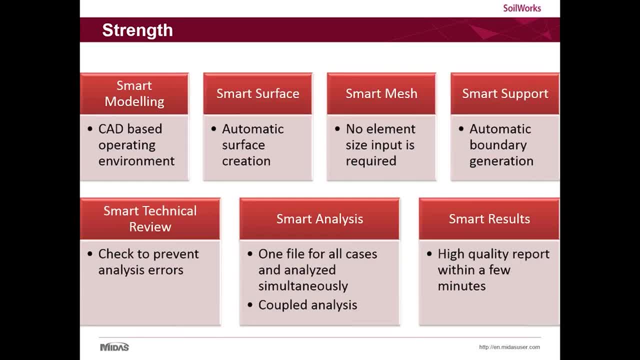 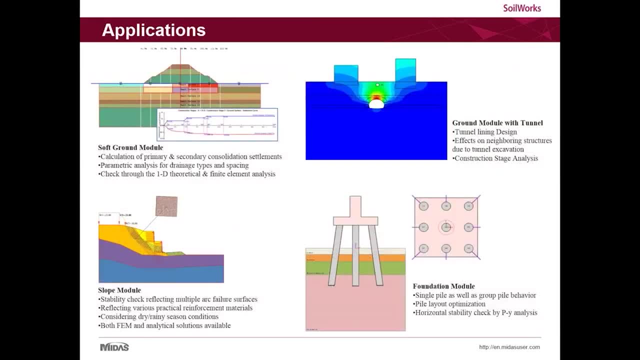 The last smart feature is smart results, where we can extract high quality report within few minutes. Some of major project applications of soil works are mentioned here: Soft ground module. using this we can obtain primary and secondary consolidation settlement results. Parametric analysis can be performed for various drainage types and spacings. 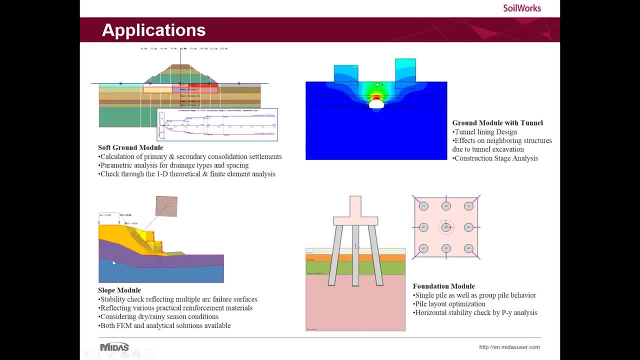 One day consolidation analysis can be performed. Next is ground module with tunnel. Using this module, we can perform tunnel lining design effects on neighboring structures due to tunnel excavation construction stage analysis can be performed. The next is slope module, in which multiple arc failure surface can be reflected for slope. 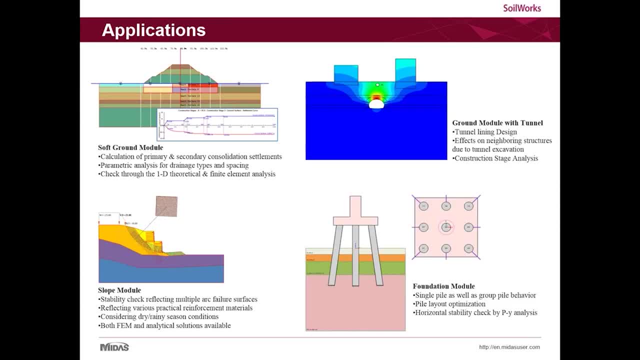 stability analysis and various practical reinforcement materials are supported in soil works which can be used. Both dry and rainy season conditions can be considered. Finite lament method, along with analytical solutions, are available in soil works. There is foundation module as well, in which single pile as well as group pile behavior. 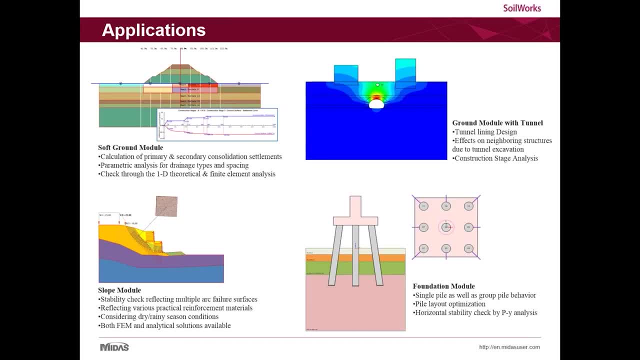 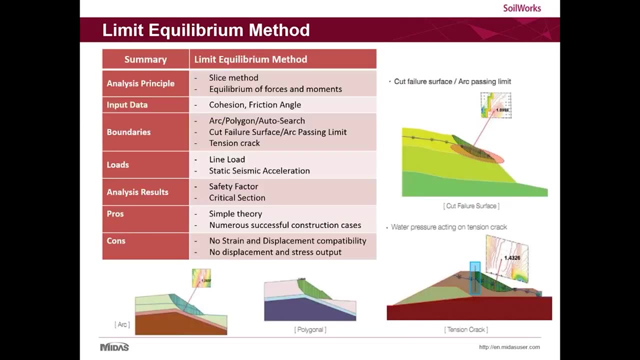 can be simulated, Pile layout optimization can be performed And horizontal stability check by PY curve extraction can be performed. Now lets discuss limit equilibrium method. On your screen you can see a summary of limit equilibrium method. It is a method of slices in which the failure surface is divided into numerous number of. 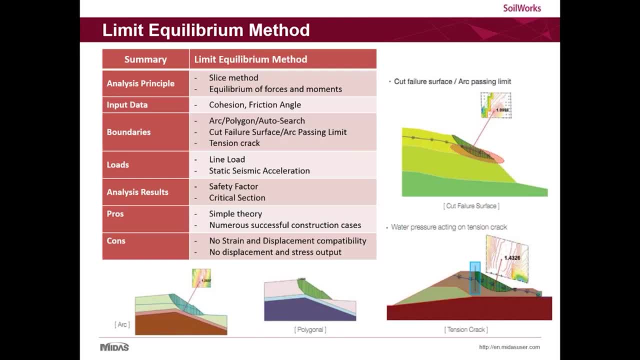 slices and equilibrium of forces and moments is checked for. the slope stability calculation calculation Input data for the ground layers is cohesion and friction angle. Boundaries defined in Soilworks are arc polygon. auto search Arc is actually shown on the bottom left corner In this. users specify the nodes, or we can say centers, using which various 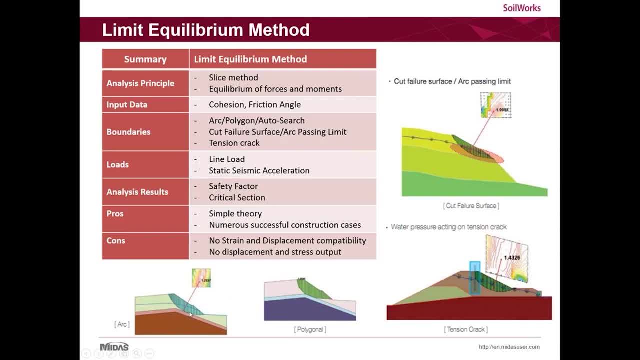 failure circles will be drawn and factor of safety for every circle will be calculated. The other option is using polygon, in which the users can specify a polygon itself, onto which the factor of safety will be calculated. Third option is auto search, in which we can automatically search for most critical failure surface and we don't need to define the 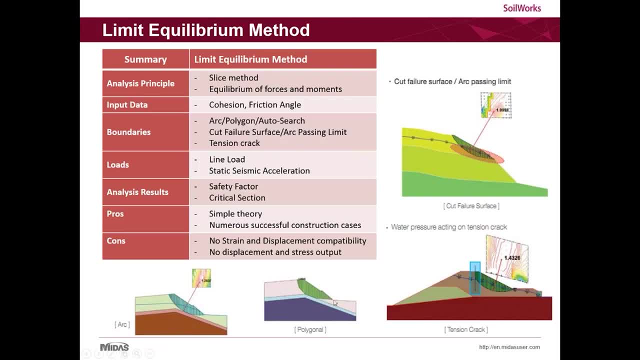 centers or the polygon. There are other boundaries like cut failure surface or passing limit. These are only used to limit the number of circles or the polygon generated in ambient soils. Soilworks also supports tension crack, Tension crack. Considering tension crack, what the 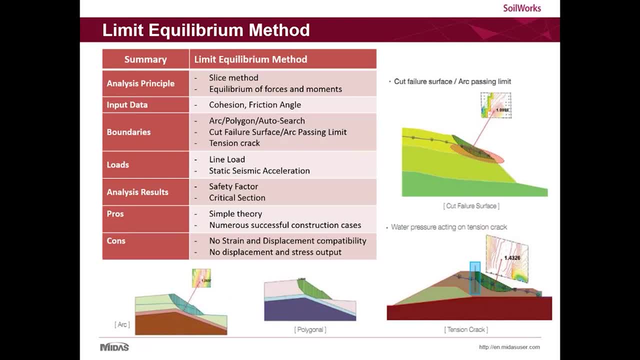 software does is the slices having tensile normal force are exerted to make the surface check. What the software does is the slices test the natural forces that are tensile. MARGE of two work-ppa is located in the absolute specific point to the right-hand corner in. 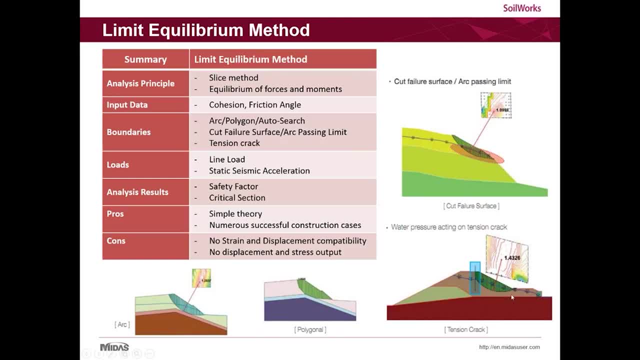 the十-meter lens For a total force of scans in the area where the plot is by this color. the value is utilizzable guests complete science. These tests are dominated by field- and solar data. The ignored for factor of safety calculation, As you can see in the image on bottom right. 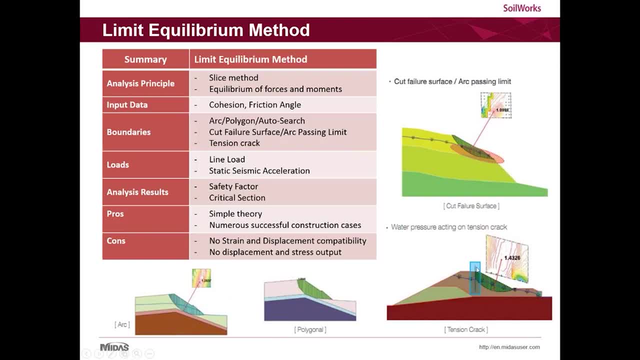 this is the location of tension crack, highlighted in the blue rectangular box. Beyond the tension crack, the slices are not considered for factor of safety calculation. That is more accurate FOS calculation. The loads which can be defined in soil works are line load and static load. 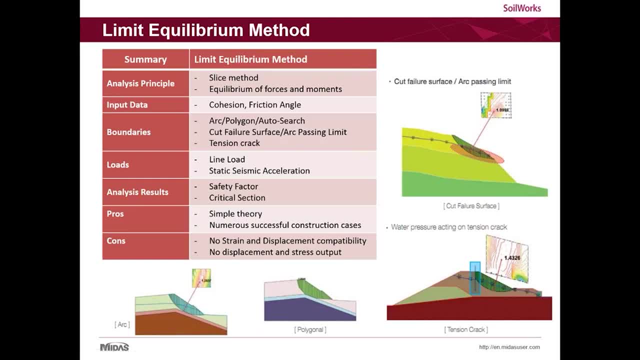 and seismic acceleration load Analysis results available in soil works are factor of safety and the most critical failure section. Advantages of using limited equilibrium method is that it's a simple theory with numerous successful construction cases, So we could say that limited equilibrium method is quite reliable when it comes to slope stability analysis. Cons. 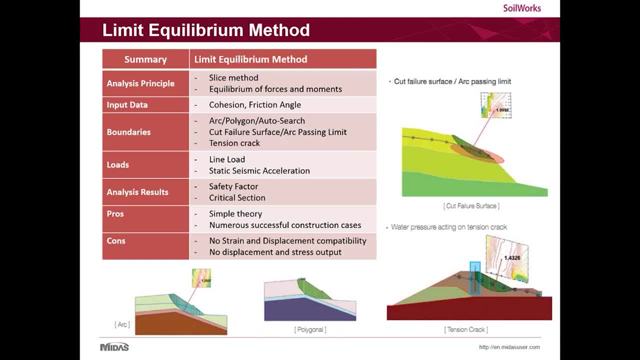 about limited equilibrium method is: no strain and displacement compatibility, no displacement and stress output. All these cons can be overcome by using finite element modeling, which is also supported in moderate soil works. but in today's session we will only be discussing limited equilibrium method. 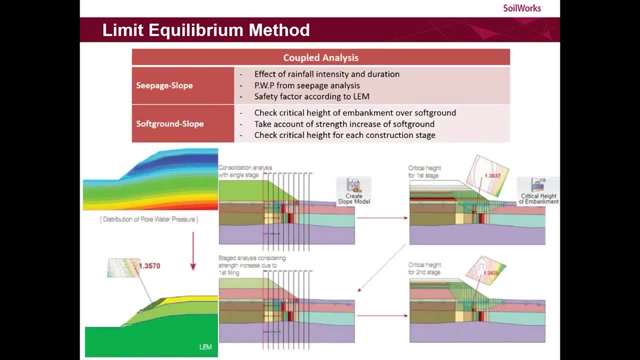 Now I will give you some information about coupled analysis in minor soil works. There are 2 kinds of coupled analysis supported by slope module in SOILWORKS. First is seepage slope. In seepage slope, firstly, what we do is we perform the seepage analysis of the ground like this shown in the top image In this. 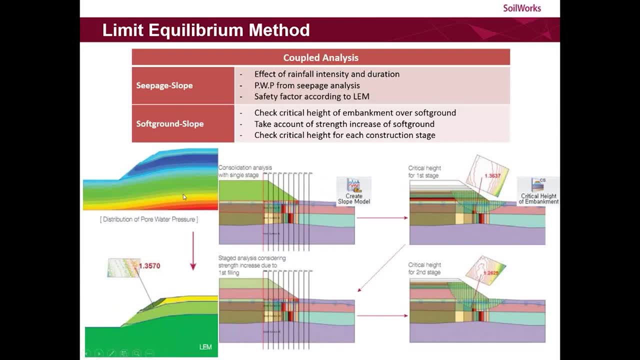 seepage analysis, the effect of rainfall intensity and duration is considered. Using that, we obtain the pore water pressure. These results are sent to limited gram method model, which is used in the slope module, and then we perform the factor of safety calculation, considering the pore water. 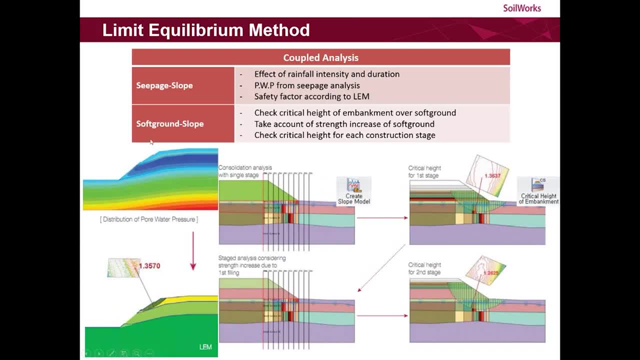 pressure results. The other coupling is soft ground and slope, where we can check critical height of embankment over soft ground, take account of strength increase of soft ground, check critical height for each construction stage. So to get all this, what we need to do is perform the construction. 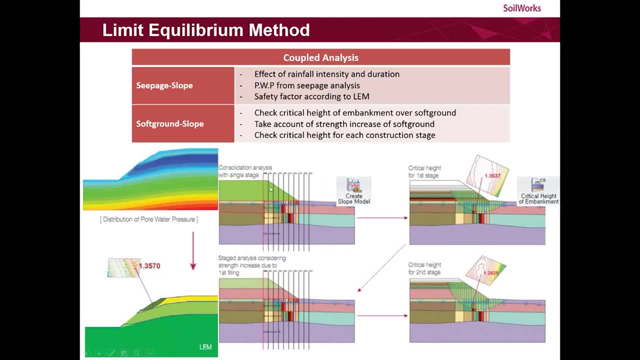 stage analysis with single stage in soft ground module get the stiffness of all these soil layers from single stage analysis. This model can be sent to slope module and then variable height of embankments can be defined in slope module and minimum factor of safety is calculated. 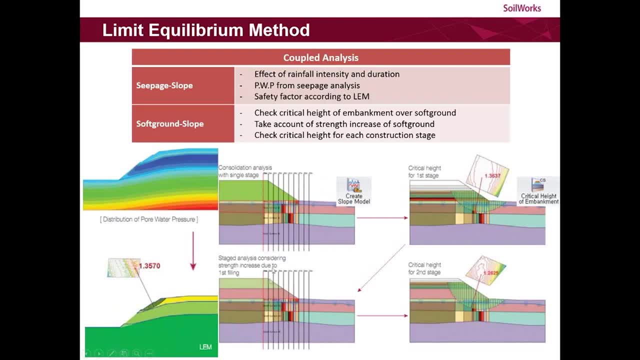 based on that, This single layer of embankment can be further divided into two parts at this particular height. After dividing the model into two further construction stage analysis will be performed and this will give slightly increased strength of soft ground, which can be further considered. 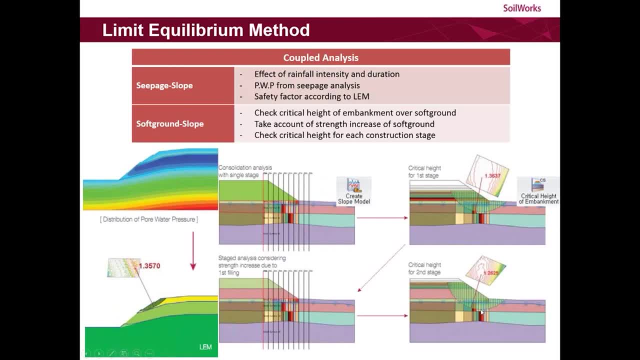 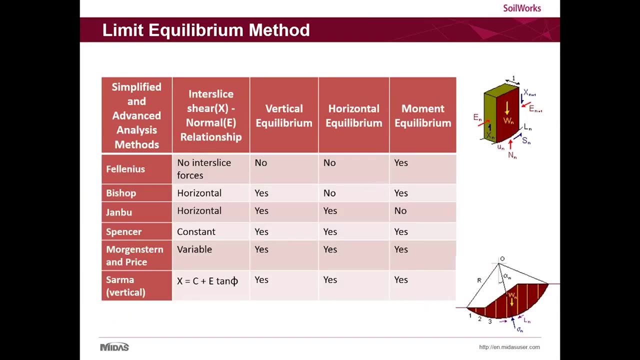 Subtitles by the Amaraorg community. So this is how iterative process works and we get all these results. Here we'll discuss simplified and advanced analysis methods supported in soil works. Simplified ones are Felinius, Bishop, Janbu. Most commonly used ones are Bishop and Janbu and are quite old. 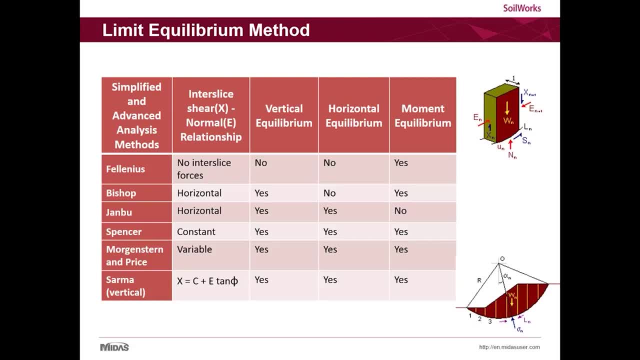 Bishop has a disadvantage that it doesn't consider horizontal equilibrium, whereas Janbu doesn't consider moment equilibrium. These are the drawbacks of these older methods. Advanced analysis methods like Spencer, MNP, Surma- all three of them- can consider all sorts of equilibrium and give much more accurate results compared to Bishop and Janbu. 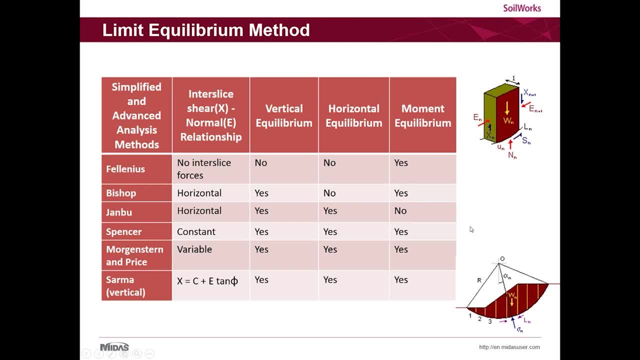 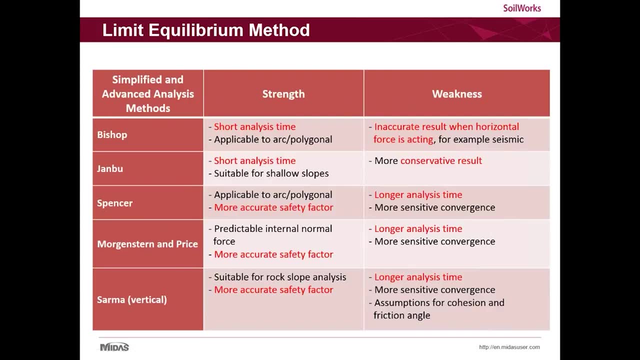 Let's take a look at the advantages and disadvantages of these simplified and advanced analysis methods. Bishop method and Janbu method, which are the simplified analysis methods, take shorter analysis time, but the result for Bishop method is inaccurate when horizontal force is acting and for Janbu. 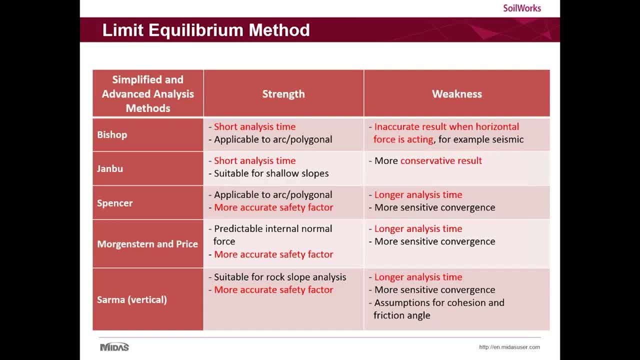 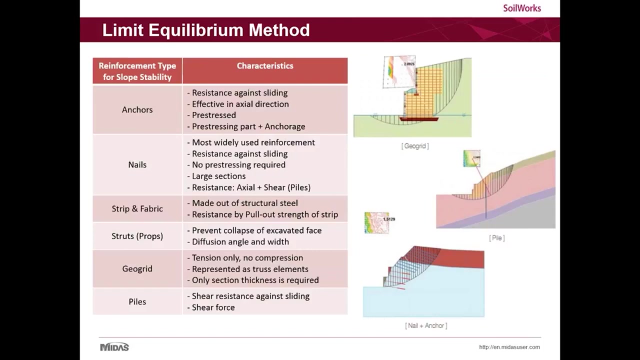 method, the results are too much conservative. With advanced analysis methods like Spencer, MNP or Surma the analysis time is quite longer, but the factor of safety calculation is more accurate and is well supported in modest soil works. After we check the factor of safety, if the slope comes out to be unsafe, we can use reinforcements. 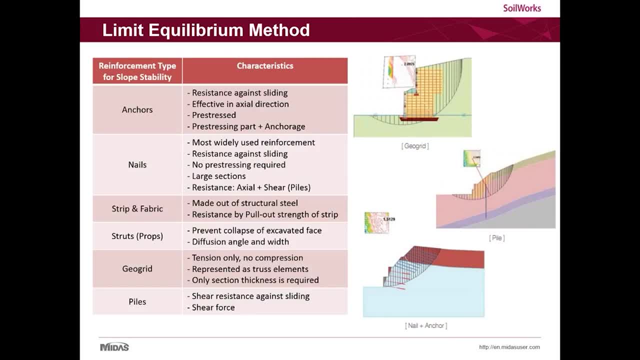 like anchors, nails or all these which are well supported in soil works. In today's demonstration, I'll be using nails, which are most widely used reinforcement and they do not require any crease tracing. Along with that, they have axial as well as shear resistance. Nails are shown in this image, the bottom right. 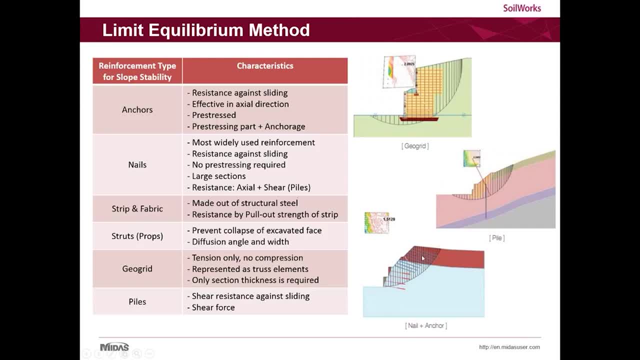 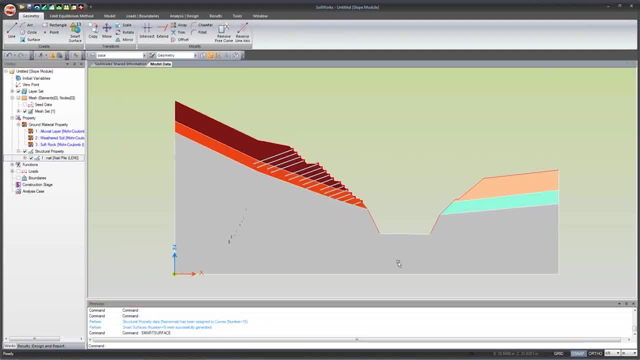 During this demonstration we'll see the application of seven smart features for using limit-examiner method for the slope shown on the left. Yet again, I will click on this and within seconds SmartSurface generates surface along all the lines. So after I have generated the surface, I can assign the ground material properties. 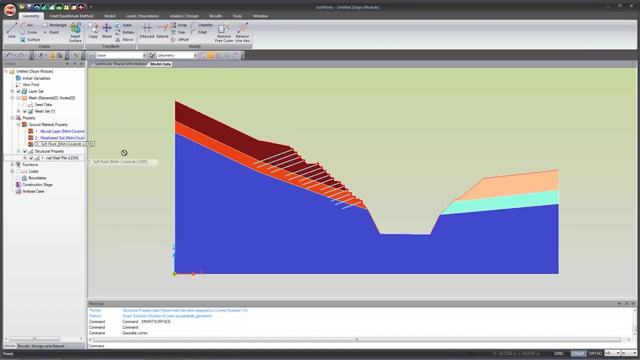 All I need to do is select the ground material and drag and drop it. I'll select the second ground layer. Select the ground material, Drag and drop. Third layer selected. So very quickly, my structure property has been defined, assigned my ground materials. 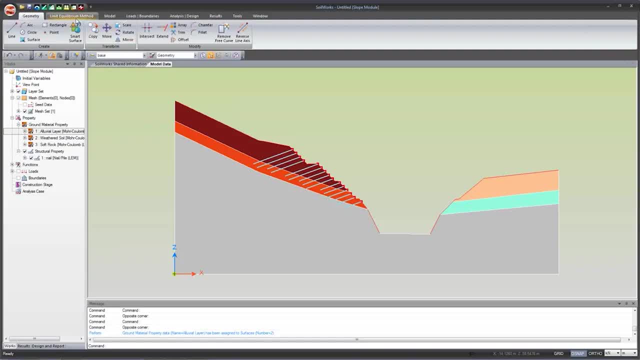 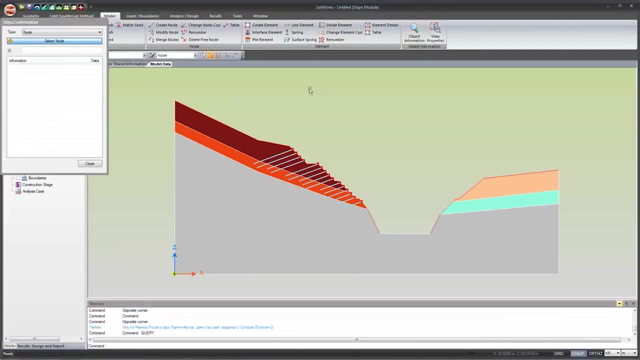 have been defined and assigned. After this I can go to model and click on object information. If I have to check anything, we can check node, curve, point, surface, anything. Surface is kind of query. so if you want to inquire something or some changes are required. 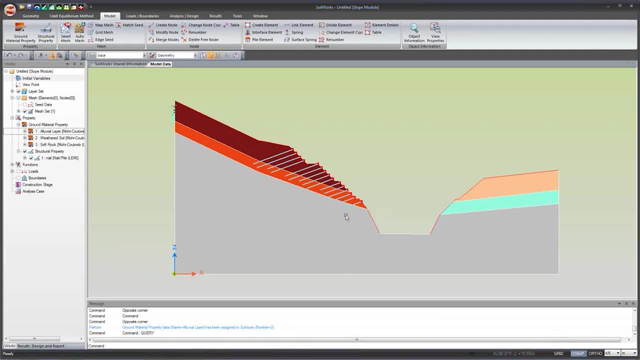 anything changed in the model is needed, so it can be done even at this stage. So that's the advantage with this software. And now I'll show you smart mesh. In smart mesh, we don't need to enter the size of mesh anywhere. 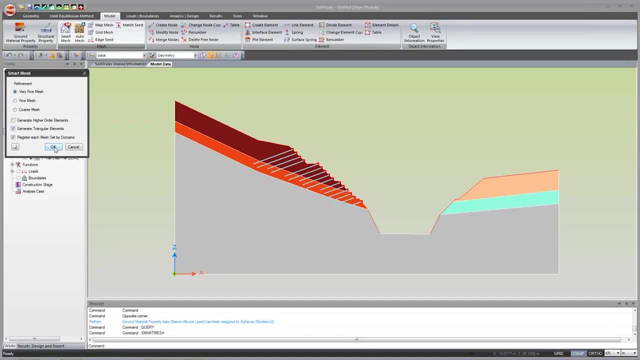 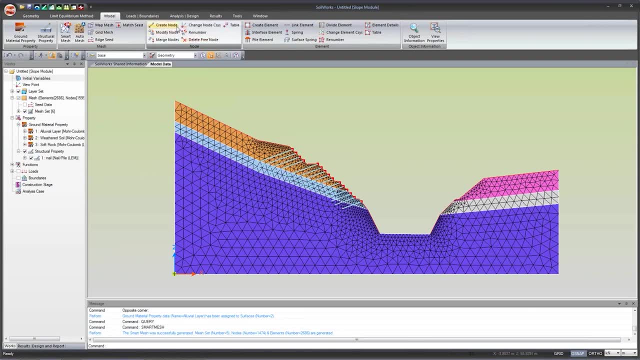 We can just choose very fine mesh with triangular elements and software will automatically generate a suitable mesh for that. And then I can click on smart support, boundaries and smart support. So just click OK and the support is generated. So it's that quick. 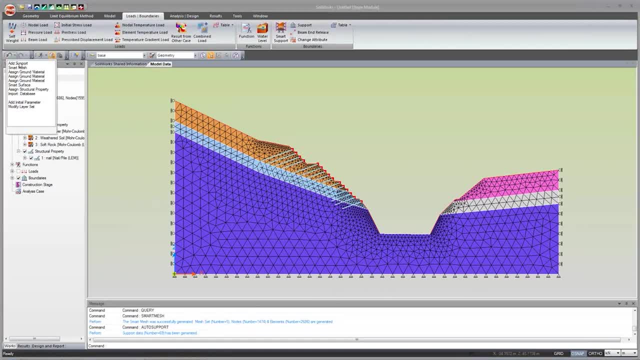 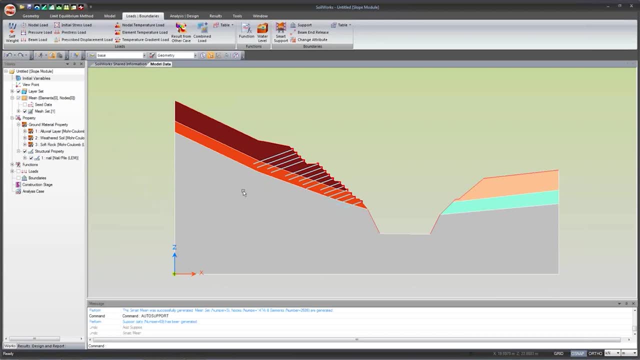 But these two smart features- smart mesh and smart boundary- are not needed for limited theorem method. So I'll just undo those steps and I'm back to the stage where I assign the ground material properties to the ground layers. Now I'll go to limited theorem method tab. I'll define the line load. I'll define distributed. 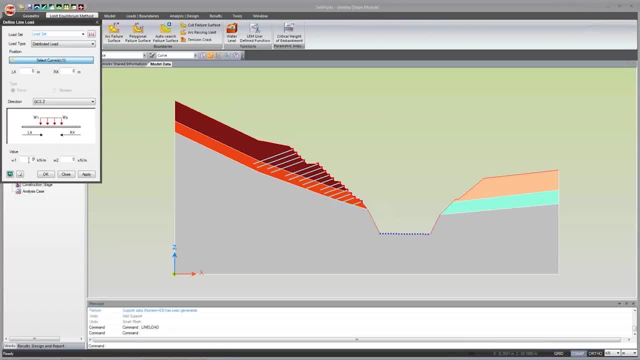 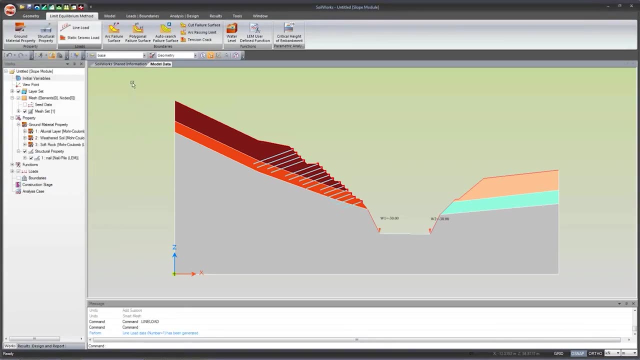 load. select a curve and enter a value of minus 30 kilo Newton meter And click OK. After defining the line load, I'll go to arc failure surface. I will name it arc failure surface. I will name it arc failure surface. 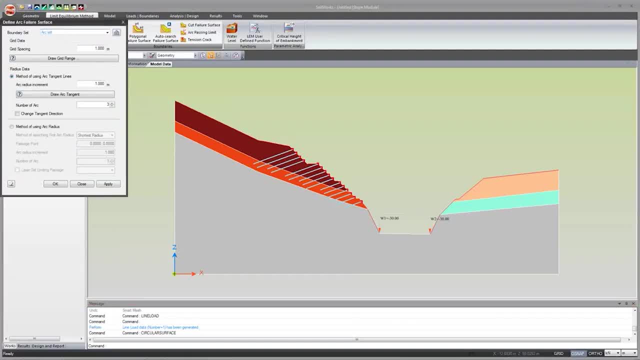 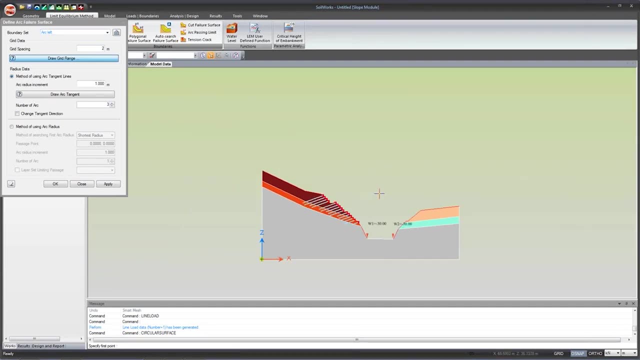 I will name it as arc left. Grid spacing will be 2 meters. I have to draw a grid for calculation of factor of safety, So I'll just minimize the model and define a grid. Let's say I'm choosing quite a big grid. 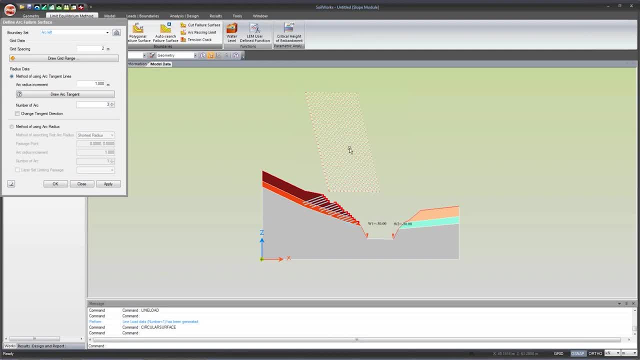 So that my- Okay, Let's see Failure circles- reference nodes do not lie outside this rectangle. I'm trying to capture maximum possible areas for the failure circle. We have two methods to define the failure arc. One is using tangent method, Other is specifying the radius values. 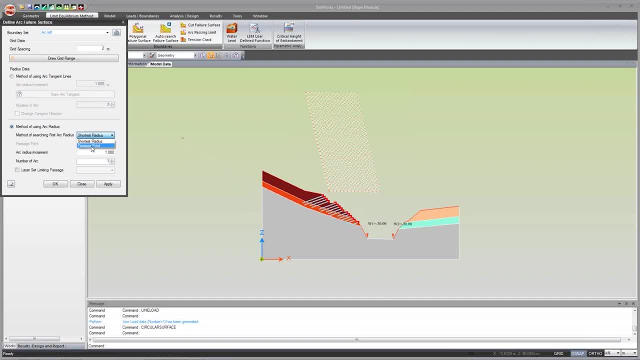 I'll choose the radius option. Now I'll choose a passage point, The first failure circle, with a 3-point line. I'll define the radius. It should be 3.5 meters is passed through this point. Arc radius increment: various arcs will be constructed, increasing. 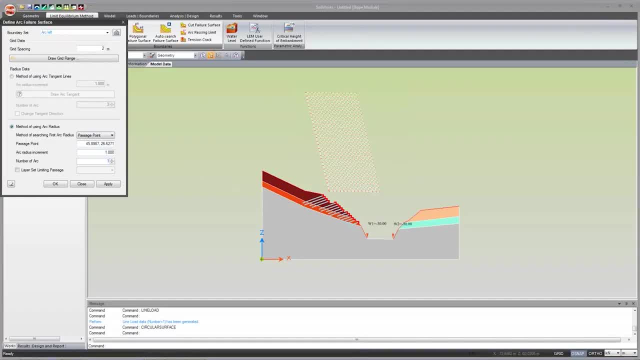 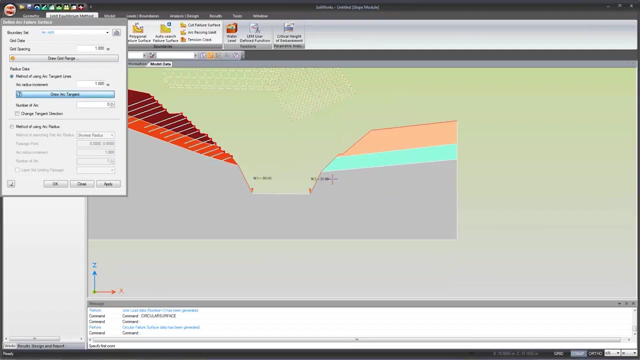 the radius by 1 meter. Number of arcs for every center will be 10 and click apply. Now I'll define the second arc, that is, arc right. I'll define a grid range here. In this I'll use arc tangent lines, So I have to define a tangent. I'll just zoom it: define a tangent. 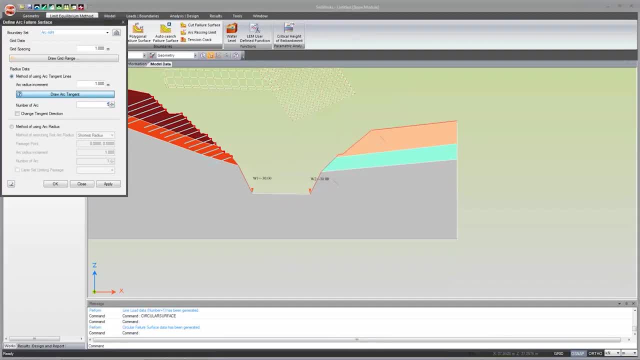 line here. Number of tangents: let's say I define 5 tangents. So I'll define a tangent line here. Number of tangents: let's say I define 5 tangents. So what the software will do is for every center it will make arcs which will be tangent. 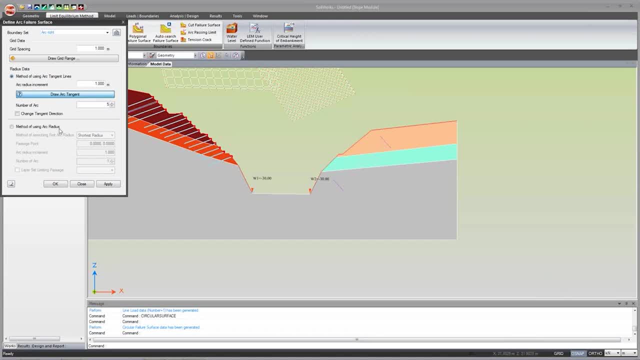 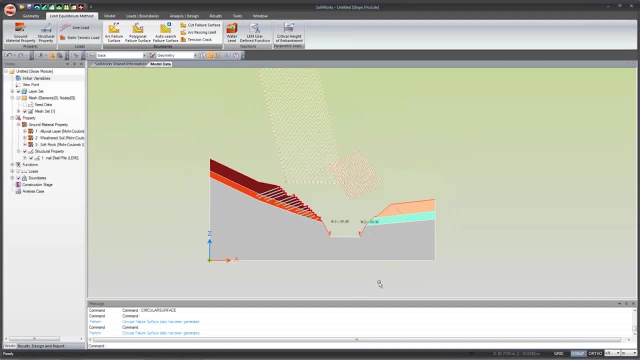 to the lines that I have defined And now I can click OK. So two arcs actually, the boundary conditions for limit equilibrium method have been defined, And after this I can go to analysis or design. tab. Design option: I choose cut slope, specifying the 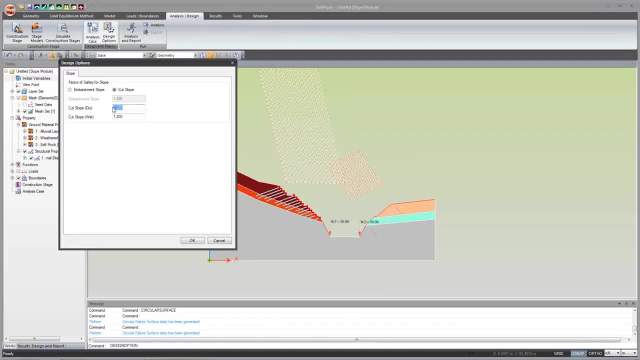 model is a cut slope. The factor of safety for dry condition is 1.5.. For wet it's 1.2 that I have chosen here. So if the factor of safety in this model file is less than 1.5, then the slope will be unsafe. since I'm analyzing it for dry condition, Now I go to 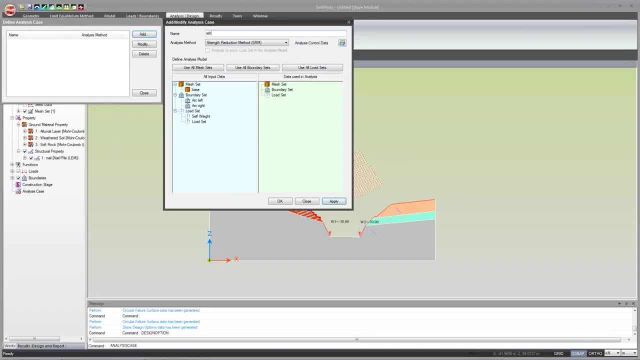 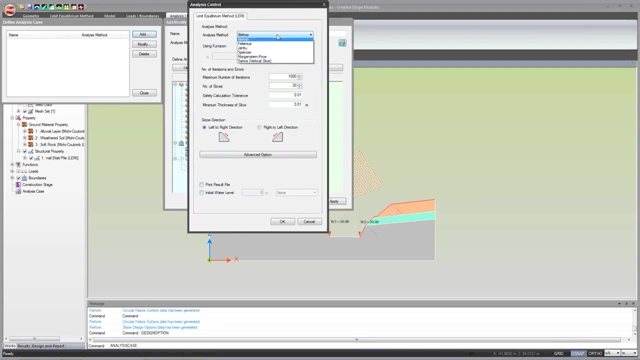 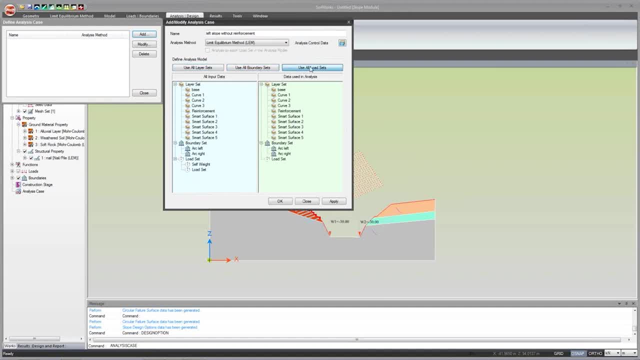 failure, click OK. All layer sets, all boundary, all load. I'll just drag and drop reinforcement to deactivate it. Drag and drop arc right to deactivate the right failure circle And just click apply. Next load case I'll generate with reinforcement. So I'll just drag and 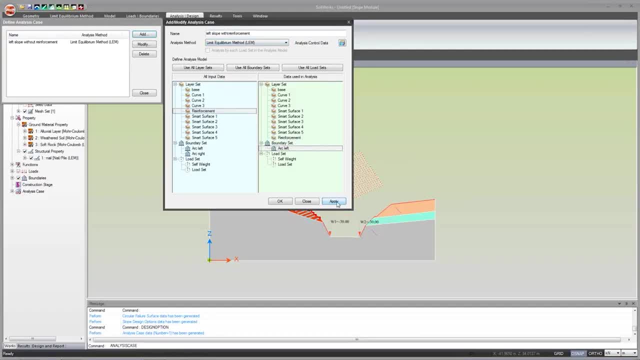 drop reinforcement again, So it's activated, Click apply And the last load case is right slope with reinforcement. Reinforcement doesn't matter for right slope because reinforcement is not at all defined. I can choose right to left failure direction. That's the only change that I need And here 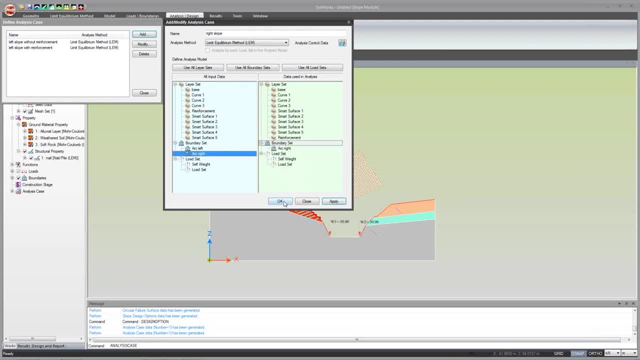 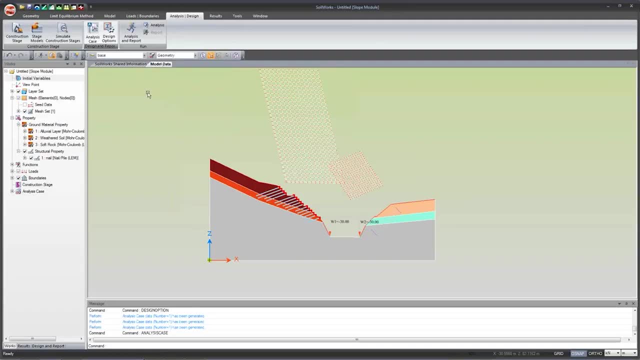 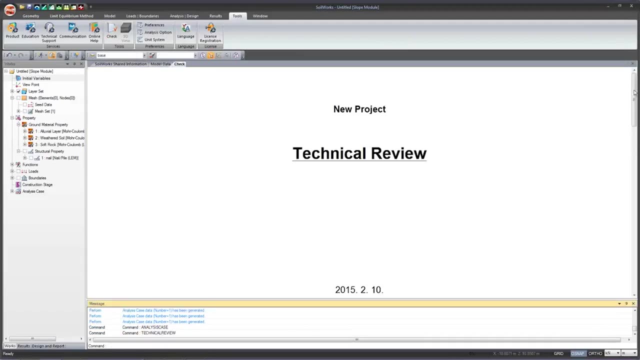 I can choose right boundary condition, Then click OK. After defining everything, I'll show you the fifth smart feature, that is, tools check. So just before running the analysis, I can have this review. This will show me all the input definitions. 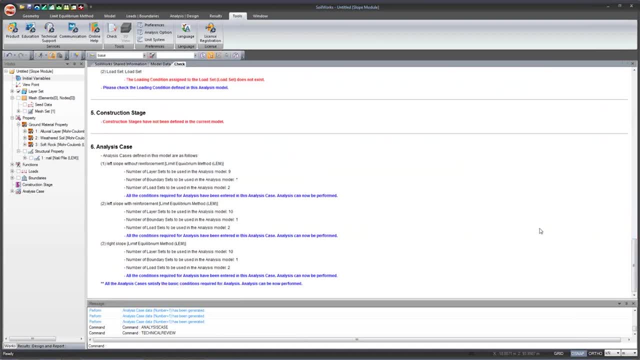 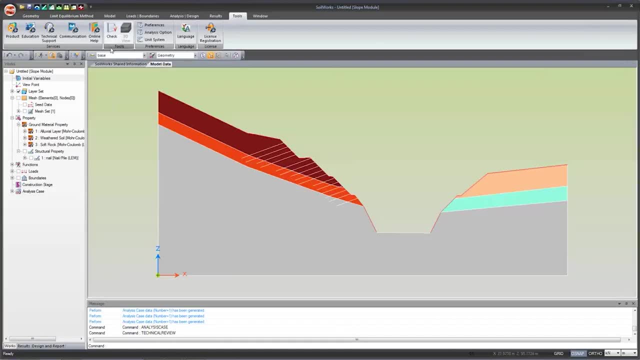 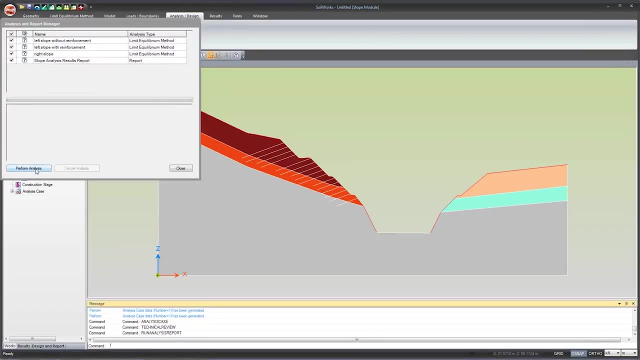 This will show me the results that I have made and if I am good to perform the analysis now or not. Analysis can now be performed for all the three cases, So I'll just go to analysis tab, Click on analysis and report And click perform analysis. I'll save this. 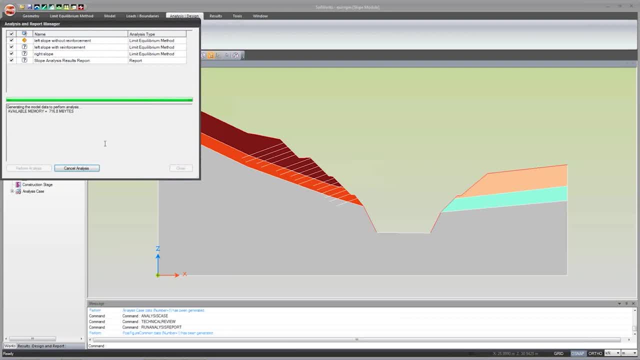 model, as say, example, And run the analysis. This is the smart analysis feature of Soilwork, So I can see the results, that all the load cases are analyzed simultaneously. I do not need a separate model file for a model without reinforcement and the model for with reinforcement. 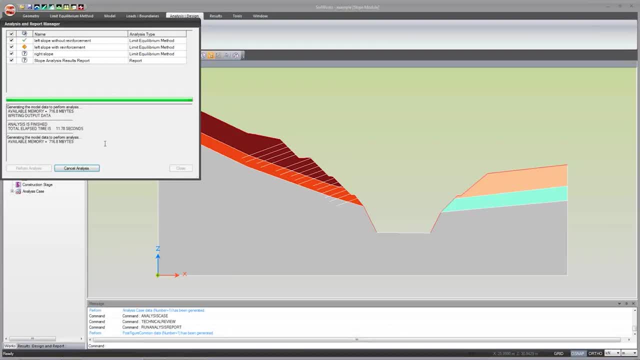 and another model for right slope. I am analyzing all the three cases simultaneously. Not only that, along with that, I'm generating a detailed design report which we will see after checking the results And you can find how helpful it is for summarizing the results. 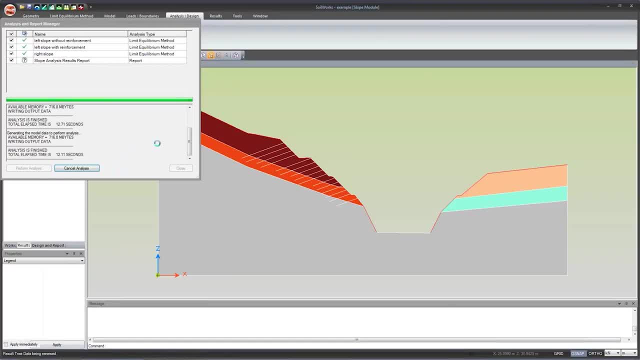 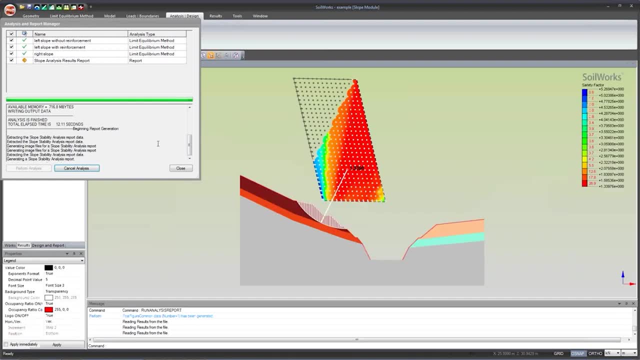 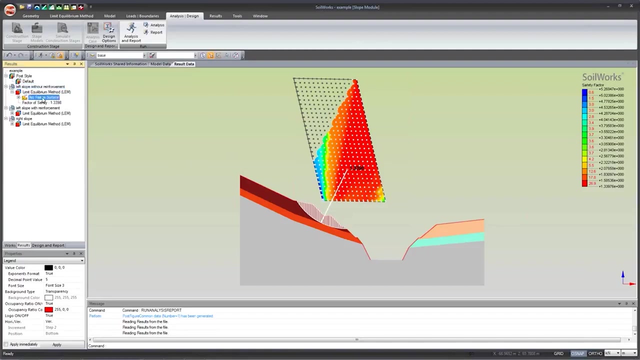 Now the report generation is starting. It will take a few minutes for the report to be generated. The slope stability analysis report has been generated now I can close it and now check the results. The factor of safety without reinforcement is 1.3398.. 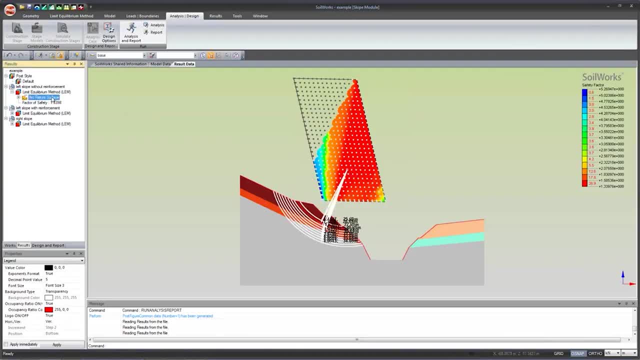 I can see all the failure circles just by clicking on this. The factor of safety with reinforcement is increased to 2.3316, which is as expected. so 1.33 is less than 1.5, so there was a requirement of reinforcement, and reinforcement stabilizes. 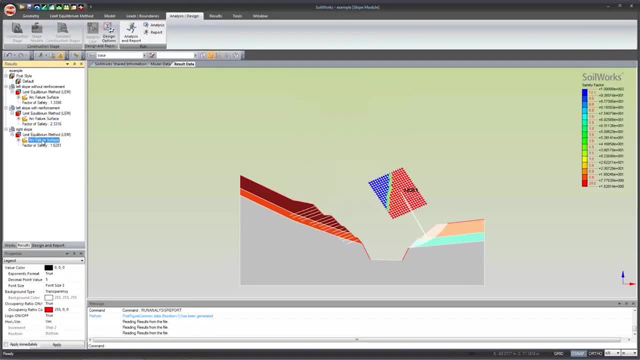 the slope. For the right slope, the factor of safety is 1.6281,, which is greater than 1.5, so no reinforcement definition is required. We can check the slice force details. By the way, the slide is not a slide. it is a slide. 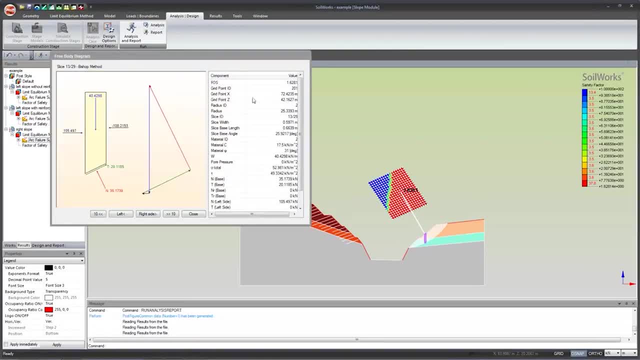 Just by double-clicking on the slice and this is the detail of the slices, and the forces in the slices can be seen here. I can just keep on changing the slice. you see, this is the slice which is highlighted and the forces are displayed here. 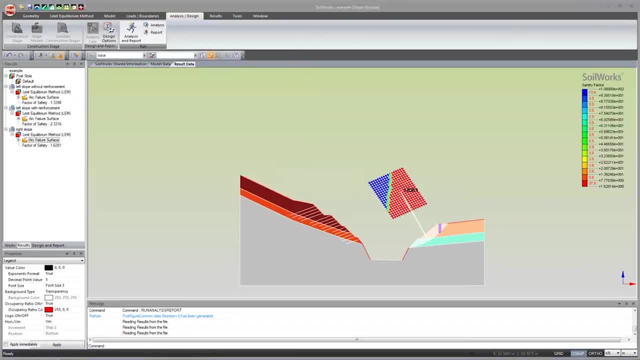 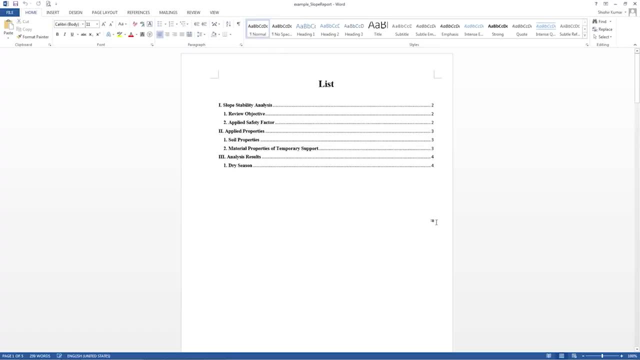 After looking at this, I'll show you the report. This is the design report which is generated. Firstly, this is the design parameter which I defined For dry season, the factor of safety should be greater than 1.5.. This is the material input with cohesion and friction angle, with saturated and unsaturated. 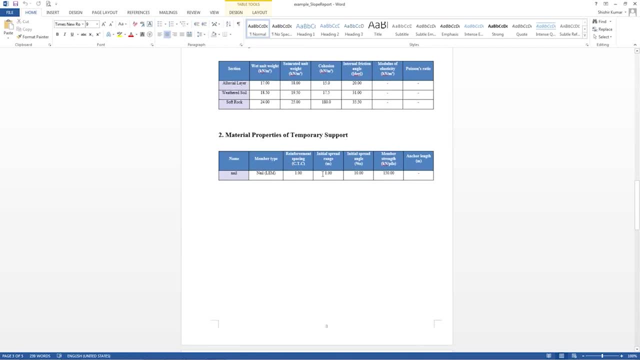 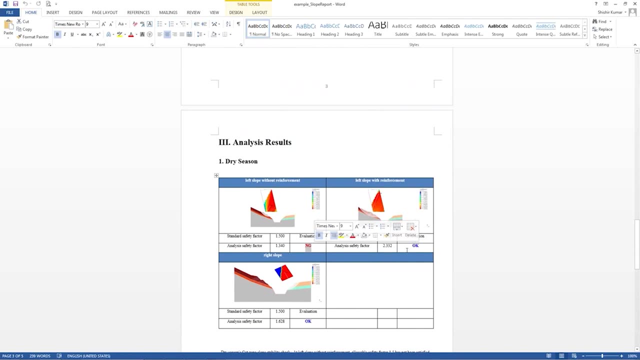 weight density. This is the structural property definition, and then this is the result. Without reinforcement, the check is not good. For reinforcement, the factor of safety is sufficient, and for the right slope, the factor of safety is okay. There is no need of any kind of stabilization. 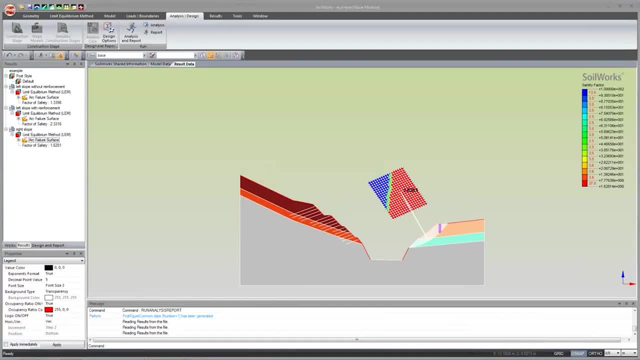 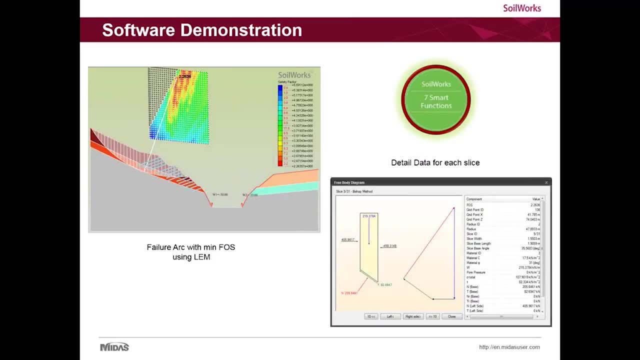 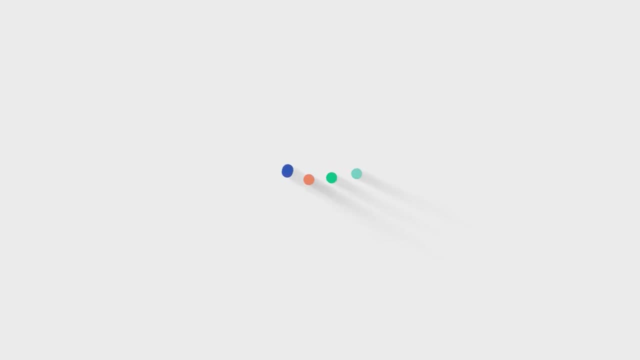 This completes the presentation of mine. I'll move back to the presentation now and I'd like to end the session. Thank you, Thank you. Thank you for watching. Thank you for listening, Thank you for watching.